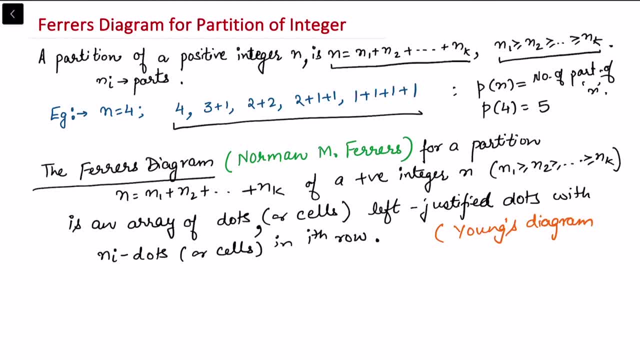 we call this as a Young's diagram, otherwise we may conveniently call this as a Ferrer's diagram. This is an array of dots or cells left, justified dots, with ni dots in the ith row, and for each partition we can represent n1 plus n2 plus nr. So this is an array of dots or cells left, justified. 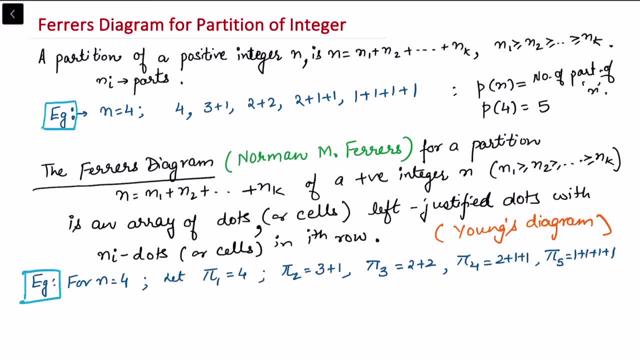 dots with n1 plus nr, So we can write it as a Ferrer's diagram. So now to understand this Ferrer diagram, let me to take the same example for which I have written the partitions. So we consider n is equal to 4 and there are 5 relevant partitions corresponding to 4.. So I have named 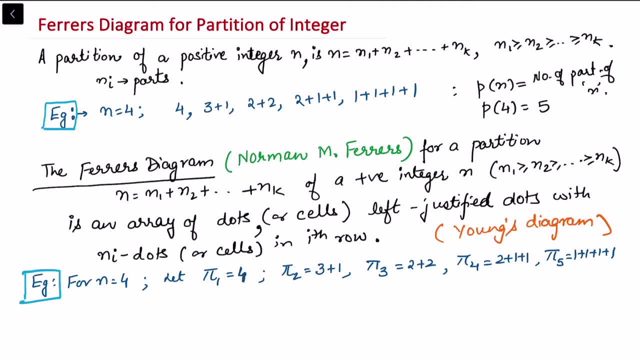 these partition: pi 1, that is 4. this is one of the relevant partition. then I have named another partition, pi 2. this is 3 plus 1. I have. I have named another partition, pi 3, 2 plus 2. similarly, pi 4, pi 5. this is just a name of the particular relevant partition. Now say I want to write an. 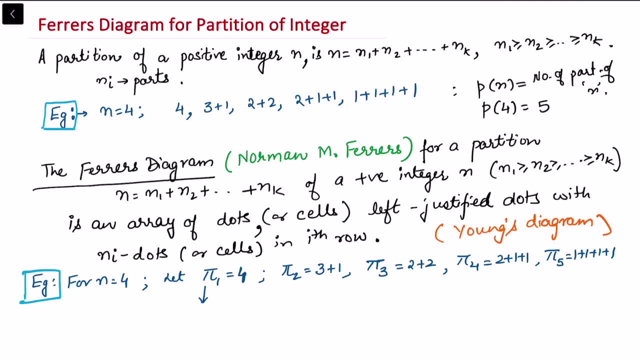 draw the fairer diagram corresponding to this one. the definition says there has to be ni dots or cells in the ith row, so in the first row, since there is only one element, one number here, so corresponding to this, i will pick up the four dots: one, two, three, four. so these are the four dots and 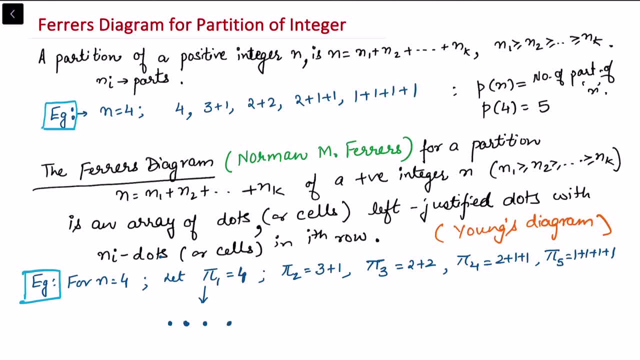 these dot have to be left aligned. so in this case there is only one part, so this becomes the fairer diagram. so let us write the fairer diagrams. this is the fairer diagrams that i'm showing here now for the next partition, pi 2, there are two parts, so this means in this notation there are: 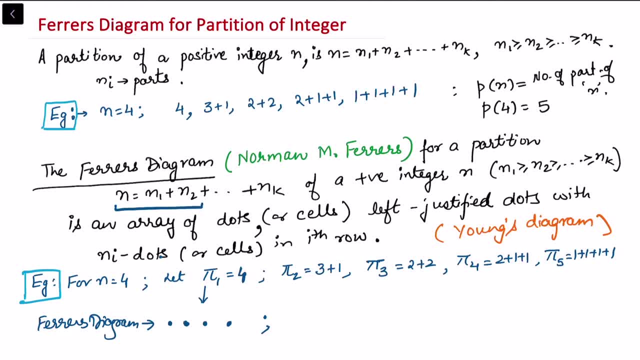 n1 and n2 and in ith row there will be ni dots. so in the first row there will be three dots and in the second dot there will be n2 dots. so we have to pick up from the definition. the first row have three dots, so this is one, two, three and the 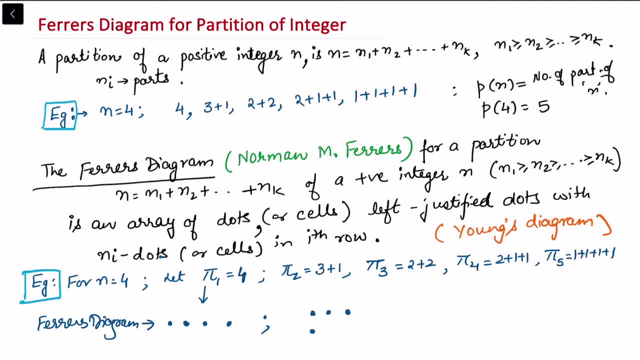 second row have only one row and we notice that these are left aligned. so this is the left alignment. so in this case you can see that this is left aligned. every dot start from the left alignment. so this is what do we mean by left aligned, so we can just draw it here also this: 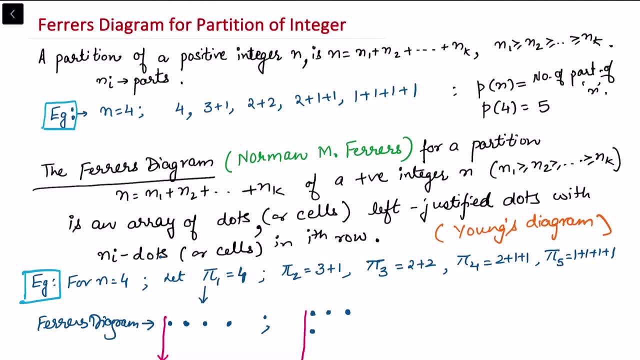 is what we mean by left align. now, similarly, in the next case, pi 3, if i want to write the perez diagram corresponding to this one, what will be pi 3? this will be 2. so here it will be two dots in the first row, and then again in the second row. also there will be two dots. 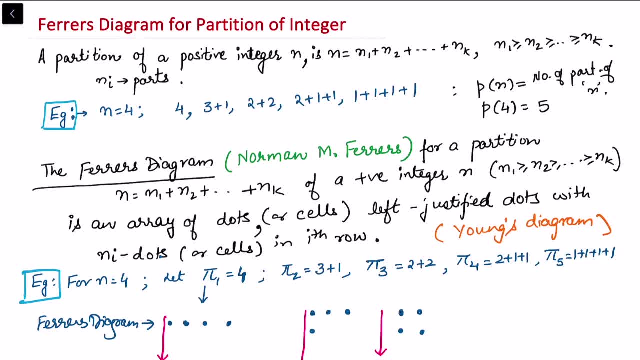 now for the next case. so let me to just take a bifurcation so that there is no confusion about the dots. so for the pi 4, first row, have two dots, the next have one dot. that's the value for n1. this is the value for n2 and then the 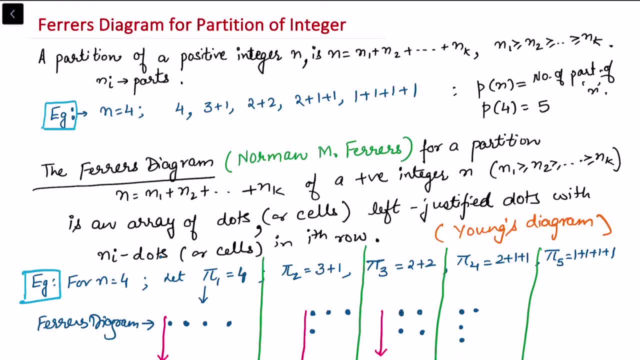 value for n3. so we will have one more dot and this is how we are making it as left aligned. now for the last case: each n1, n2, n3, n4, their value is 1, 1. so first row, have n1 dot, that is 1. 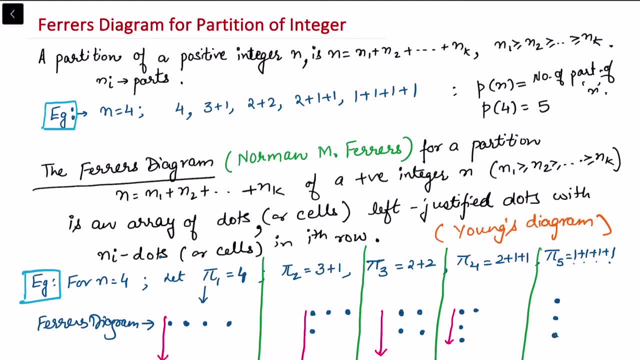 second row have n2 dots, that is, 1. third row have n3 dot whose value is 1, and fourth row have 1 dot. this is this, so this becomes the left aligned. now this is what do we mean by the ferrous diagram corresponding to the partition, and for each relevant partition there is a unique ferrous. 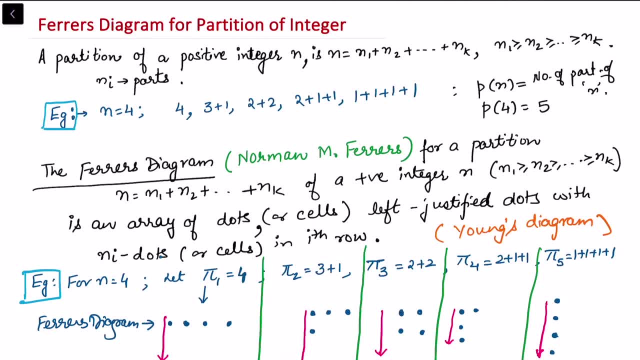 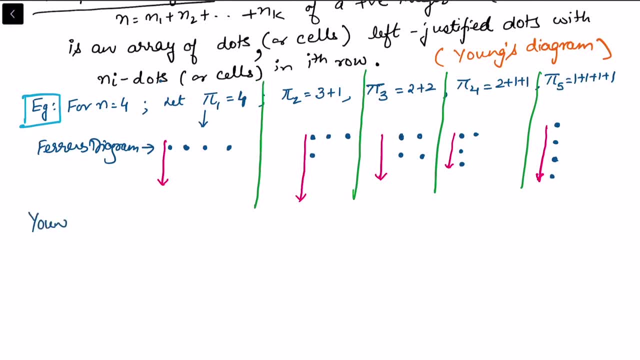 diagram. now i've also written that this is called as young diagram, in case we want to write this as a cell. so suppose, if i want to write this in the in the form of a young's diagram, so there is no much difference, except then the way we represent now, instead of these dots, what i'll do, i will use. 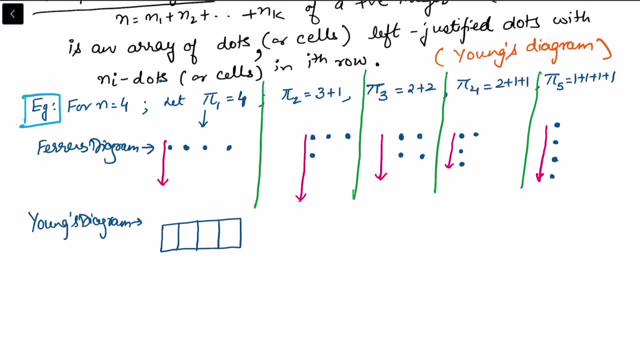 the cells so in. so it's like a square cell and then you use four cells to represent the partition four in the first row. in the second case, we will first represent three cells and then in the second row we will represent one, because the next number is one and here it was three. then, similarly, in the next partition, we will represent 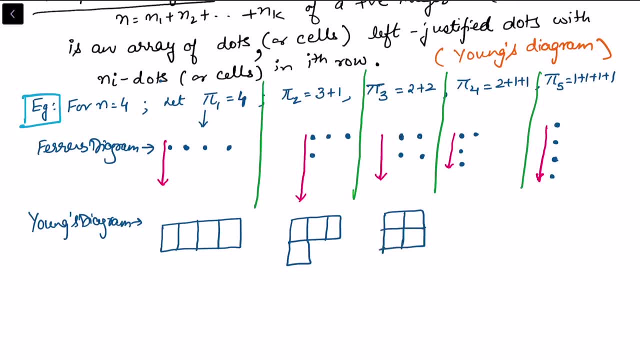 the cell two by two, so this will be two by two cell. first row also have two cells and the second row also have two cells. now, in the next case again, we will represent two cells, followed by one, followed by one more, so there will be three rows. then, similarly, in the fourth case we will have: 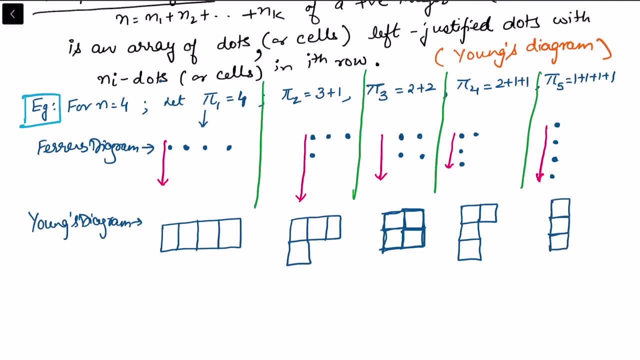 one cell, then there will be one more cell, third cell and the four cell. so this is what do we mean by the young's diagram. so this is just a representation. somebody can also show it using the x trick sign. so this is: instead of dot. we may use a strict size, so we can write it like this one: 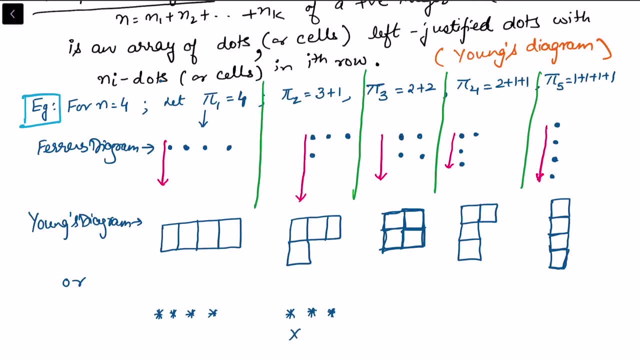 so you can have three dots here and then you can have one more dot, so everything has to be left aligned. that is this, that is the one common thing in all the definition. and then we have two for the western science. then for this case we got two dots in for the first case, then followed by one dot, and 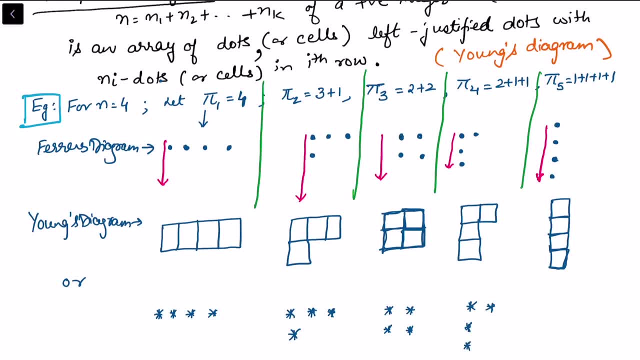 one dot and in this case everything is corresponding to one. so this is how we represent a corresponding feres diagrams, young's diagram or the definitions written in terms of any symbol, such as historic, where it fits into the definition of the ferrous diagram, it's an area of dots or cells, or a stick. 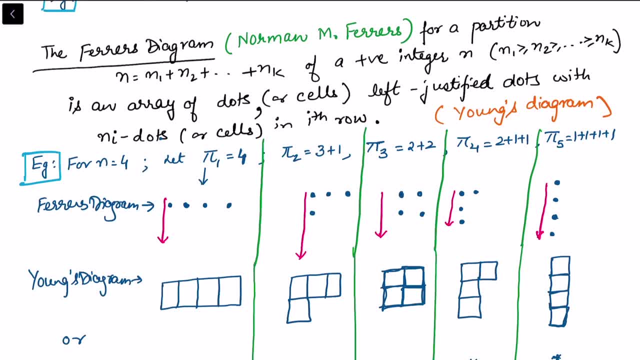 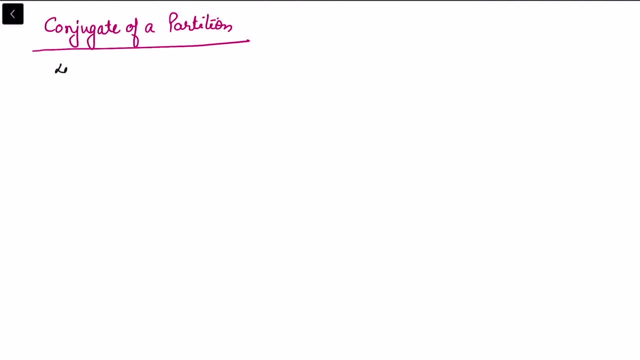 left justified dots with a straight line: Merry Christmas everyone ni dots in the ith row. now to understand what do we mean by conjugate of a partition, let me to consider a particular partition. let p be the partition of a number 15. this be a partition of. 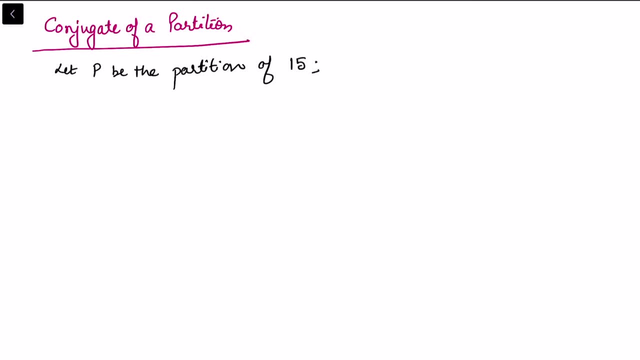 15. so p is just a notation and i'm considering p, this 15 partition, as any one of the relevant partitions: 6 plus 3 plus 3 plus 2 plus 1- and let me to write down the ferrous diagram corresponding to this one. so for this ferrous diagram, for p is this is given, as now we know that it has to be. 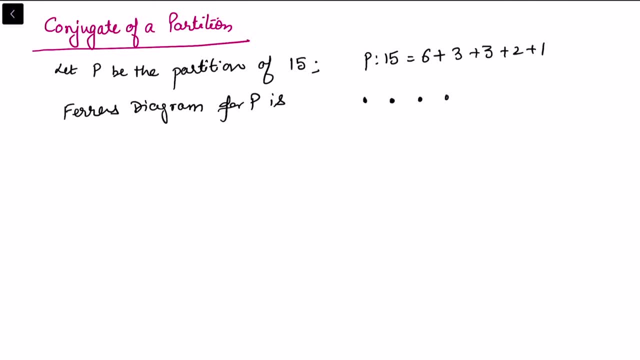 left aligned so we can have 1, 2, 3, 4, 5, 6- this is 6 dot, then we have 3 dots, and then we have 3 dots, and then we got 2, and then we got 1. so we have this left aligned diagram and to write this one. 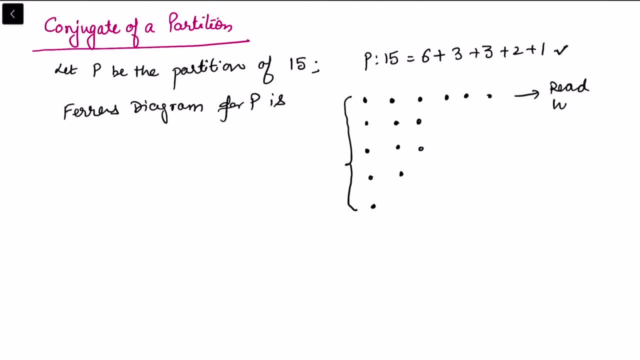 we read horizontally. basically this is how we read it horizontally to find the corresponding part. so if i read horizontally, this consists of 6 dots, then it consists of 3 dots, then third row consists of 3 dots. this consists of 2 dots and the last. 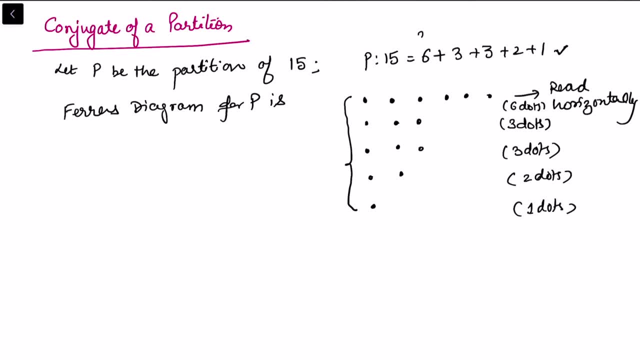 consists of 1 dot and these were actually the value for n1 plus n2 plus n3 plus n4 plus n5, and they were written in non-increasing order and this fits into the definition as i earlier defined. so i, what do i mean by conjugate? so, conjugate of p. so this i'll explain in the definition. 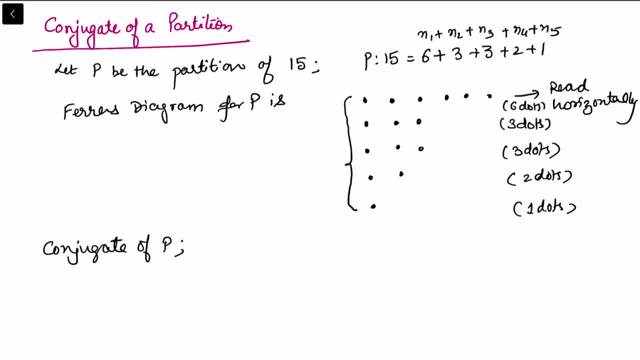 from this example, only conjugate of p means that read this diagram vertically. so now if i read the diagram, if i read the dots vertically, then we will see what partition do we get. earlier i read it horizontally. whenever we want to draw the ferret diagram, we have to keep it. 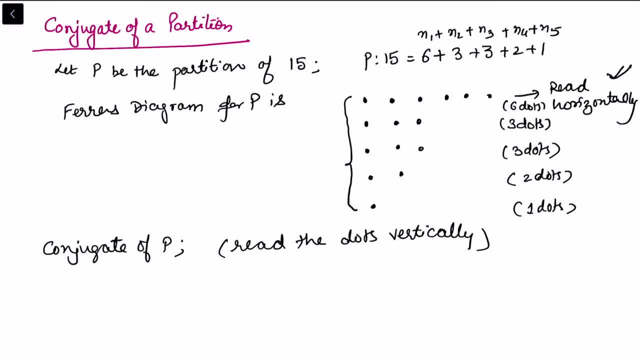 left aligned and read it horizontally. or you can say: place the dots horizontally, but now if i read it vertically, so see how many dots are there in the first column you can see. or you can simply say: in the first the arrow that i'm showing, first column, then read how many are. 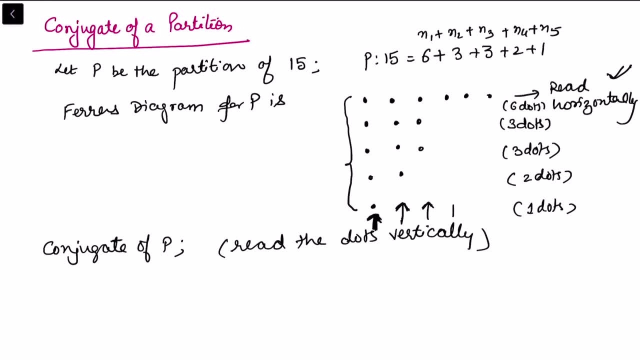 there in the second column, how many are there in the third column, fourth column, fifth column and sixth column. so you can see how many dots are available in the column. so first column, either you can read it from top or bottom, doesn't matter now if i read it this way, if i read it from the 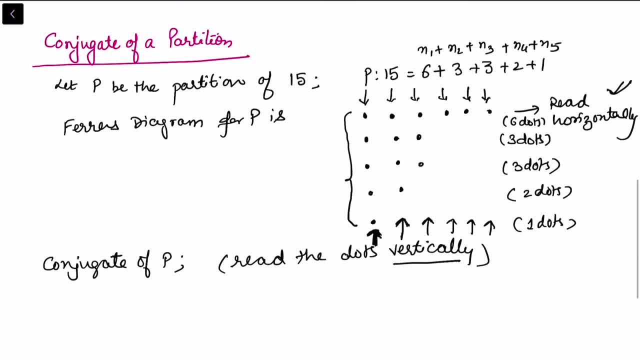 first column and if i read it vertically, then the first column consists of one, two, three, four, five. so there are five dots in the first column, followed by the next column. have four dots, followed by the next column. have three dots. then we got one dot, then we got one. 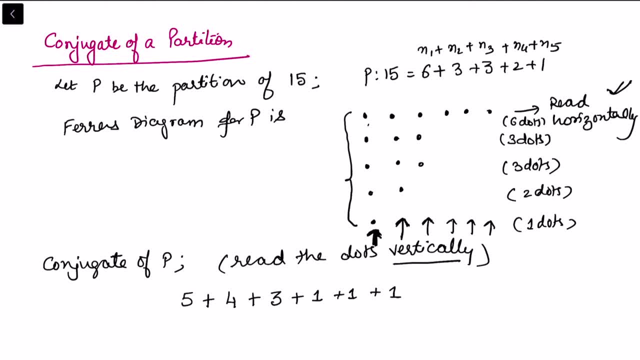 dot and then we got one dot. so this partition which we have re, which we have got from the previous case by reading the graph vertically, is what do we call it as a conjugate of p? and that's that particular partition. and we also notice that this is a partition of 15 only. so this is a 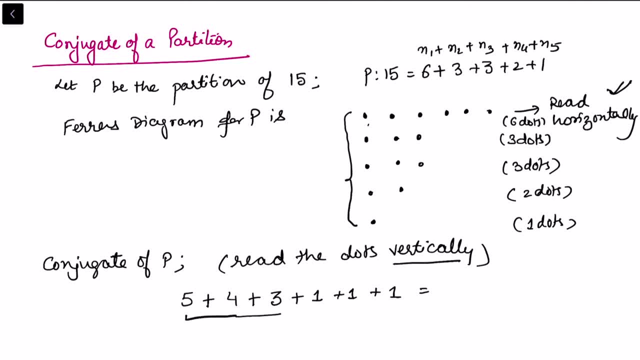 partition of 15 only: 5 plus 4, 9 plus 3, 12, 13, 14, 15. so this is again a partition of 15 only and this is also called as transpose of the ferrous diagram and we may denote it as p dash or with. 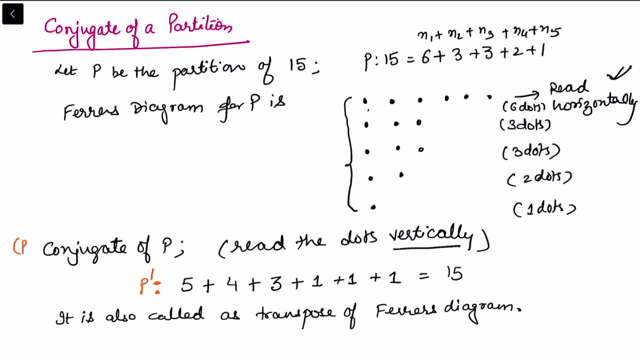 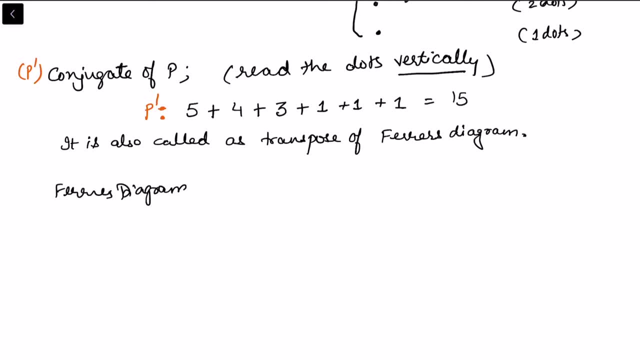 any other notations. so let me to just write down p dash. this is the conjugate of p and corresponding to this, i want to draw the ferrous diagram for the p dash. so ferrous diagram for the p dash is exactly in the same way as i've done earlier. so we have five dots in the first row, then followed. 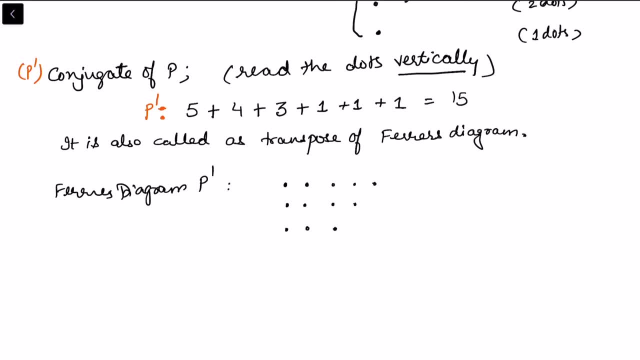 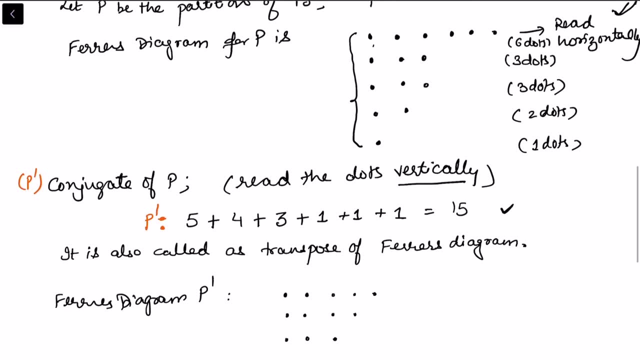 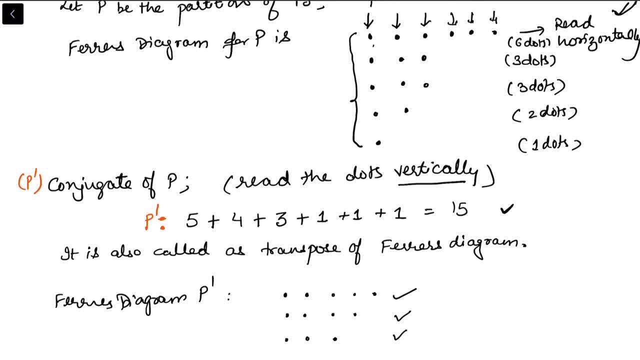 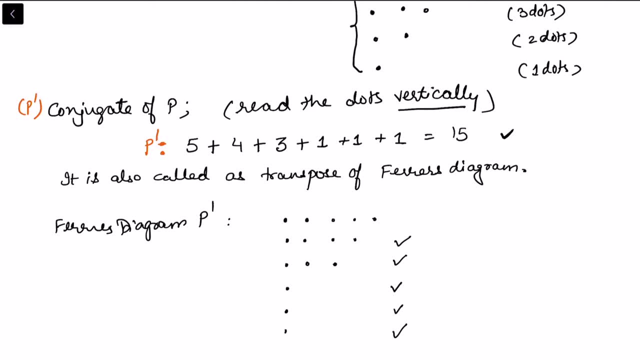 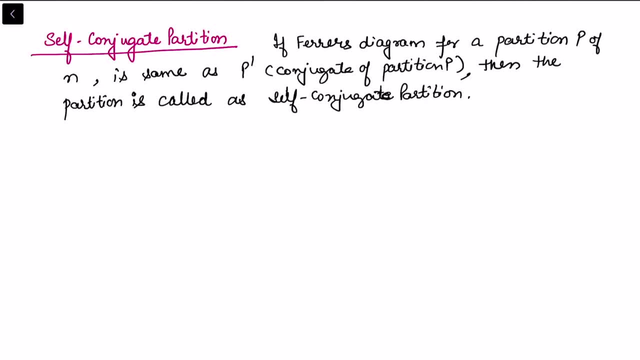 i define self-conjugate partition. if the ferrous diagram of a partition, p of n, is same as a p dash, that is, the conjugate of the partition, then that particular partition is called as a self-conjugate partition. so for this, let me to take an example. let n is equal to 4 and in this case, when i take 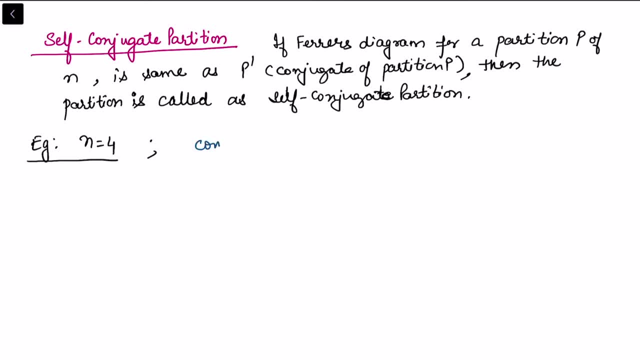 n is equal to 4. let's consider one of the partition for this. so consider p, which is equal to 2 plus 2. so this is one of the partition of 4, and if i now draw the ferrous diagram corresponding to this one, we can see this. these are the dots. so this is the ferrous diagram for the p. so for the p. 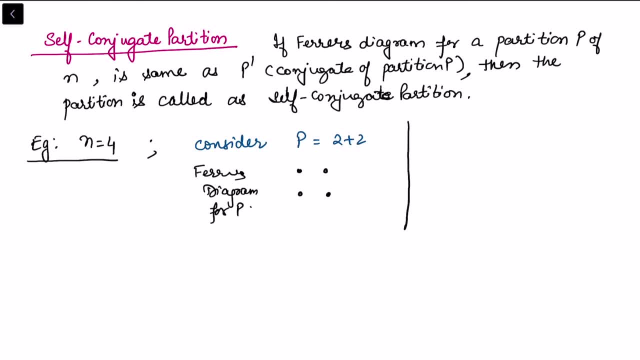 partition that i've considered. now if i take its conjugate, so suppose if i now take the conjugate p dash, and if i now read this graph vertically, then also i notice that in first column have two dots and the second column also have a two dots. so obviously for this case also the ferrous diagram will be same. so now we can say: 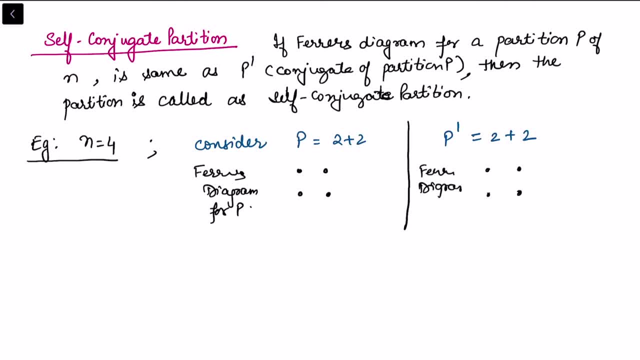 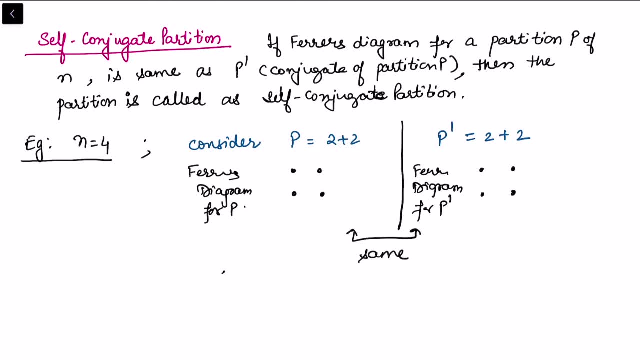 that this: this is the ferrous diagram for p dash, and we notice that both of these diagram these are same. so so 2 plus 2 is a self-conjugate partition. every partition is not a self-conjugate because they leads to different. they leads to a different partition, but in this case this is a self-conjugate. 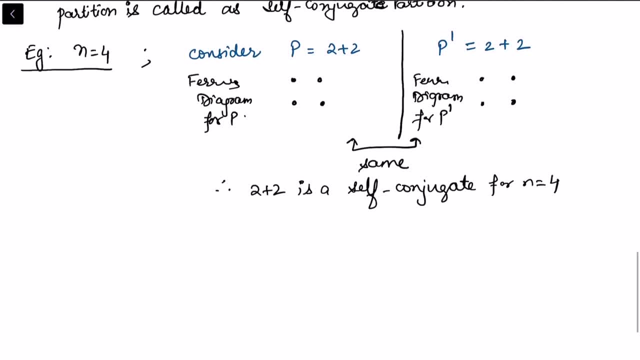 partition for n is equal to 4. we can take another example. suppose if i take n is equal to 6 and in this case say: i consider a partition 3 plus 2 plus 1, 3 plus 2 plus 1, let's say this is a partition p. 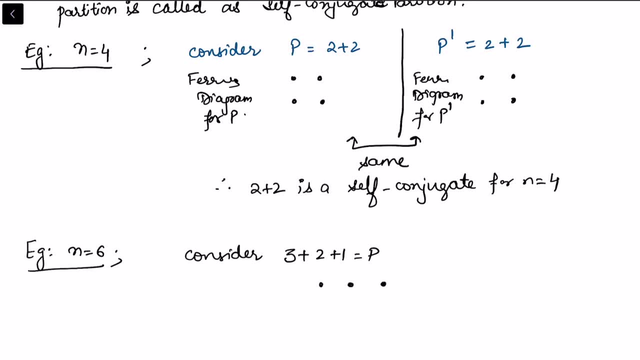 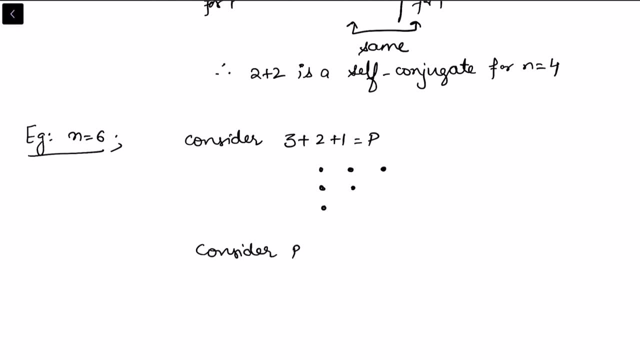 and if I draw the Ferrer's diagram corresponding to this one, this is three dots, two dots and one dot. and now if I consider p dash, so that is the p transpose or that means the conjugate of p. and then, for the conjugate of p, what I need to do? I need to read it vertically. 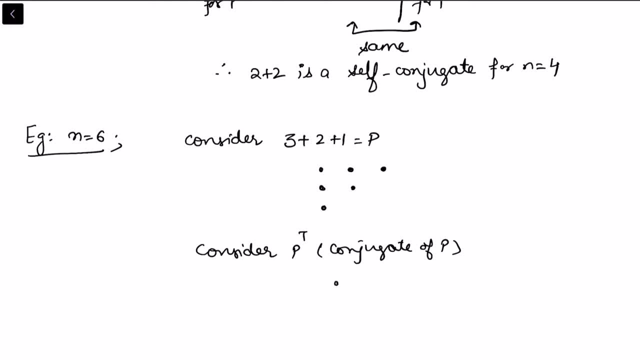 and we see how many dots are. in the first column, there are three dots. how many dots are there in the second column? there are two. and then how many dots are there in the last column? that is one. and this is exactly. both are same. so we can say that the three plus two plus one is a self-conjugate. 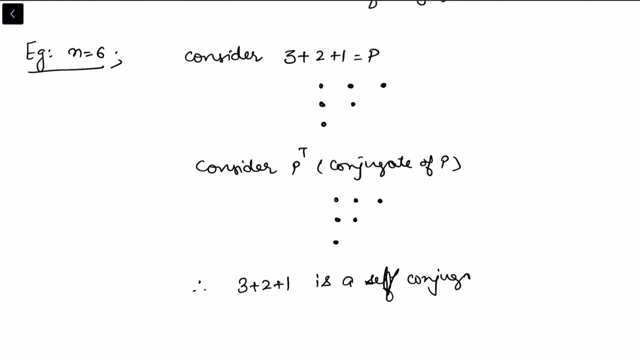 this is a self-conjugate partition of this is a self-conjugate partition of six. now let's take another example. say, if I take, n is equal to five and, corresponding to this, I consider a partition three plus two. in this case, what will be the Ferrer's diagram corresponding to this one? 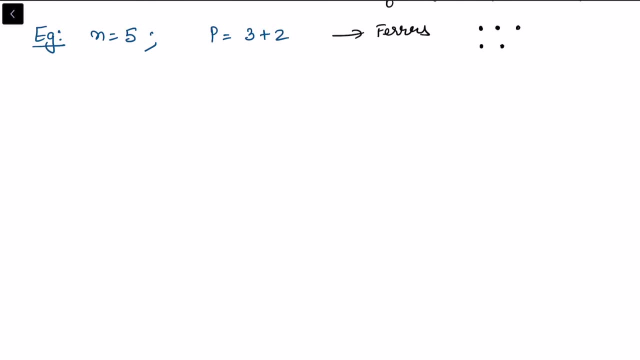 we. we need see that 1, 2, 3 and then we have two dots and if i take its p transpose, so what will be the corresponding p transpose for this? if i read it vertically, so this will lead to a partition: 2 plus 2 plus 1. now we notice that this is also a partition of 5 and earlier also it was a partition. 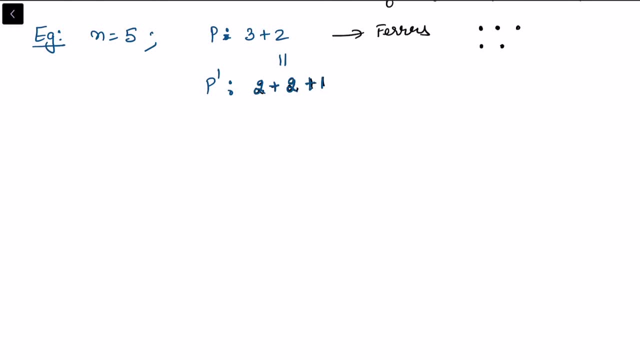 of 5, but they both are not same. these partitions are not same because the first one n1 value is 3 and in this case n2 values 2. here n1 plus n2 plus n3, there are three parts and their values different. so we can say that 3 plus 2, or you may say 2 plus 2 plus 1. these are not the self-conjugate. 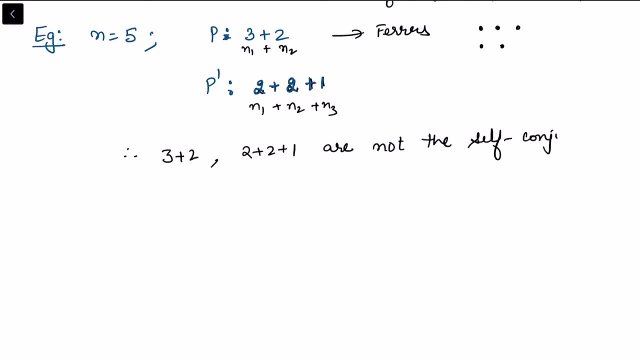 partition. so self-conjugate partition are those partition whose, when we take the transpose, they lead to the same partition. these are not self-conjugate partitions of 5. so now we use the ferrous diagram to you prove this theorem which is due to eiler. and this proof we call it as a combinatorial proof, since 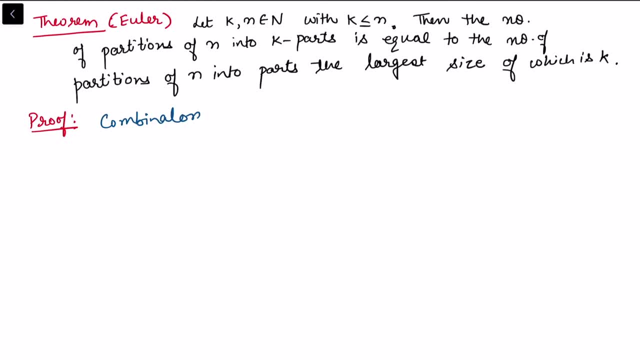 we are not using any analytic identity, although in my last videos i have used the generating functions to prove some of these such type of the identities, and so those are called analytic identities, but here i am going to use a ferrous diagram, so let's look at the definition statement. 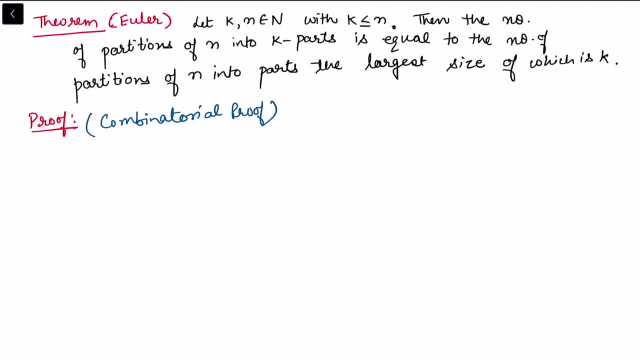 of this theorem. it says: let k and n belongs to capital n, with k less than or equal to n, then the number of partition of n into k parts is equal to the number of partition of n into parts, the largest size of which is k. so on one side we consider the partition of n into k parts, so we consider the partitions of n into k. 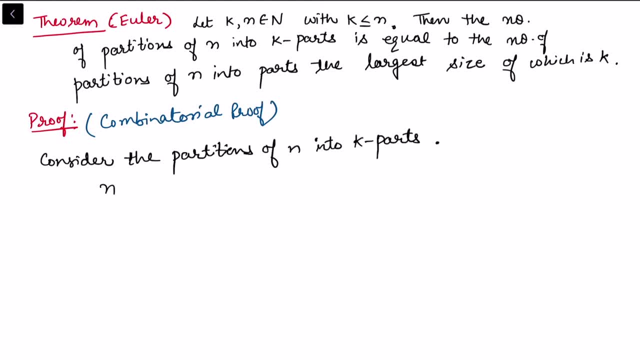 parts. so here this means i can consider a particular partition of n- and let me to call this as a particular partition- as pi, and this is a partition of n, where we need to consider this into k parts. so by definition we already know that n1 is greater than equal to n2 is greater than equal. 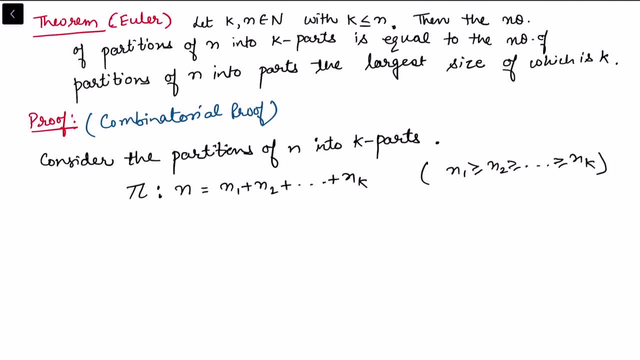 to. we can write the parts in a non-increasing order. now we notice that using the ferrari diagram. so once we draw this ferra diagram, so what will we get? ferris diagram means the first row will have n1 dots, so let's say this is n1 dots that we are having, and the second row will have 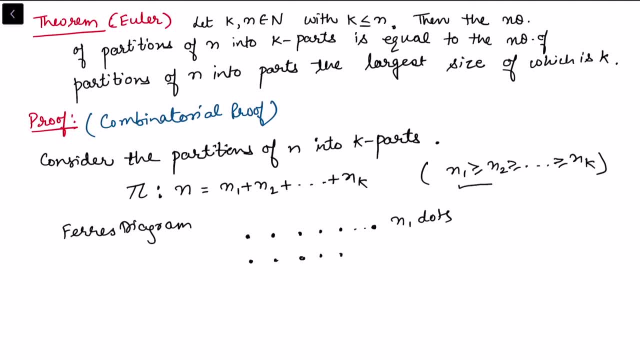 n2 dots. so now either the n2 is equal to n1 or it is n1 is strictly greater than into, so without a loss of originality we can just draw it dots here, or maybe you can just draw till the last of the dot. doesn't matter, we just call this as a n to dots and we follow the similar pattern and then 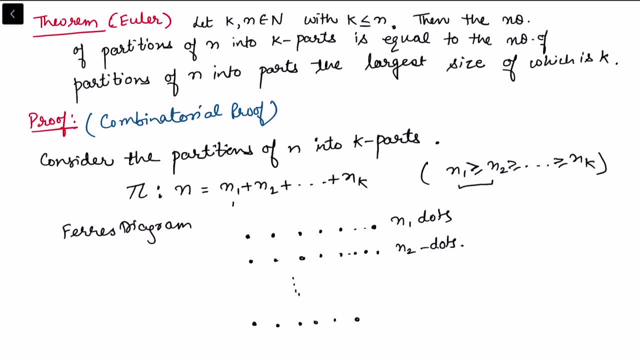 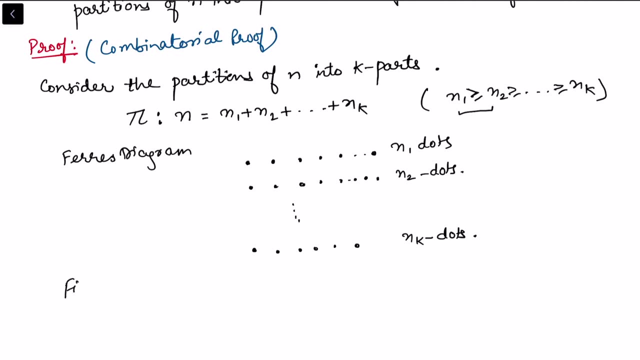 we will have the kth row because we know that there are k parts. so this means there will be k rows and the last will have k dots. so we have drawn the ferrous diagram. now what we do is we find its conjugate. so find conjugate of above partition, conjugate of above partition and in: 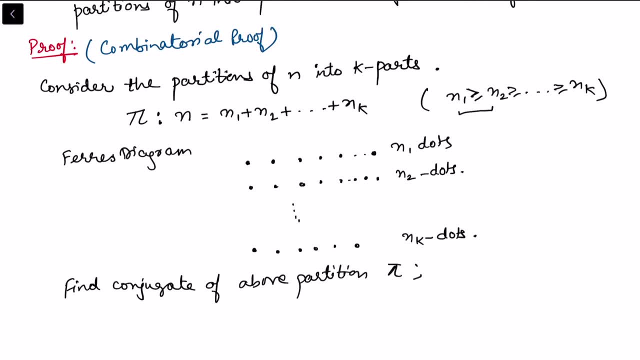 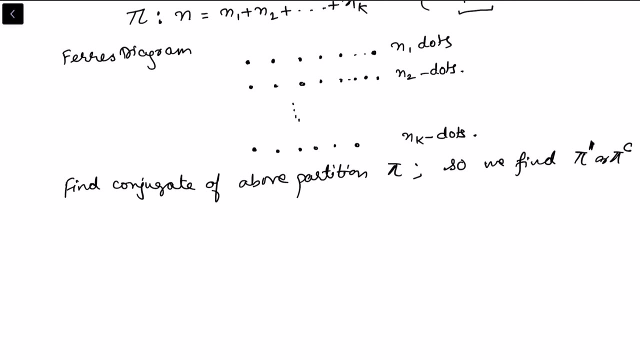 this case my above partition is pi, so let me to call. so we find pi dash, or sometime we can call this conjugate as pi c. also, pi dash stands for transpose, pi c stands for conjugate. so now, when i find the conjugate of this, we notice here how many 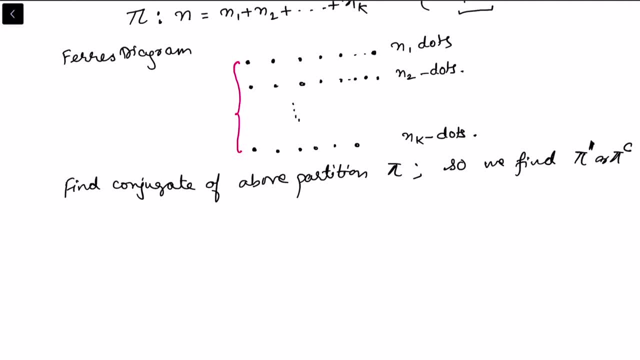 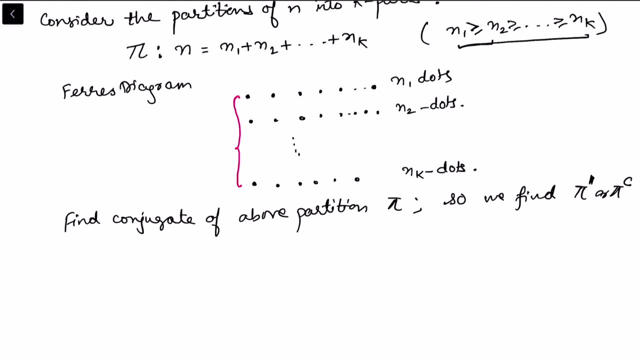 the, the, the, the. these are left lines and if and as per that definition, every n case, since we are using the partition of a positive integer, these n? i's are positive integer. that means every left aligned row will have at least one dot. so this may be. it is possible that the last part value is one. 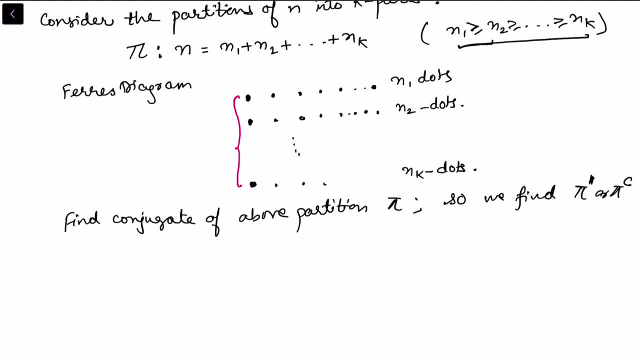 and that one dot has to come in here. so there is no, there is. this is not possible- that the last row have not even a single dot. if this is the case, then we will consider this partition into k minus one part. when we say that nk has a value, this is kth dot. that means at least one dot must. 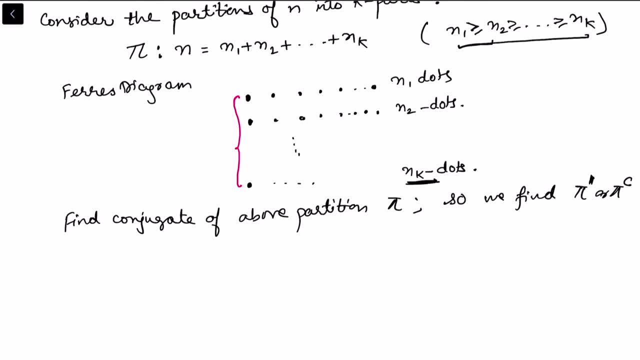 be present. so now, when i count it as vertically, or when i say when i consider its conjugate, this means the first, it will create another partition of n and in that case, the first one, this is the largest part, and this value will be k, because there are k dots. so, since there are k dots, because k dots, 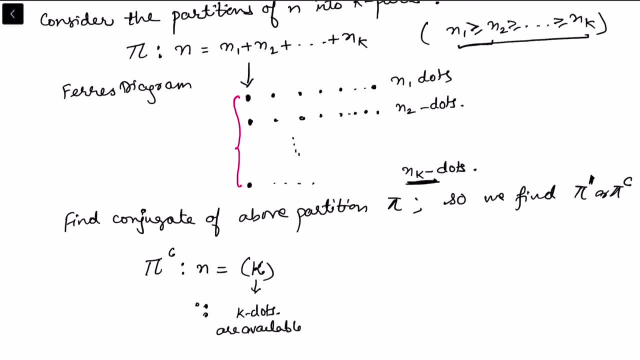 are available. these are available in first column, so when we read it vertically we see there are k dots available in this one plus. then we can have the corresponding. so let me just call this as the value n1 dash, and then we have n2 dash plus n3 dash plus 1. 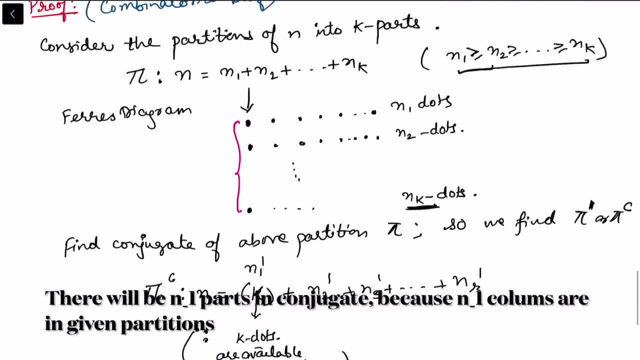 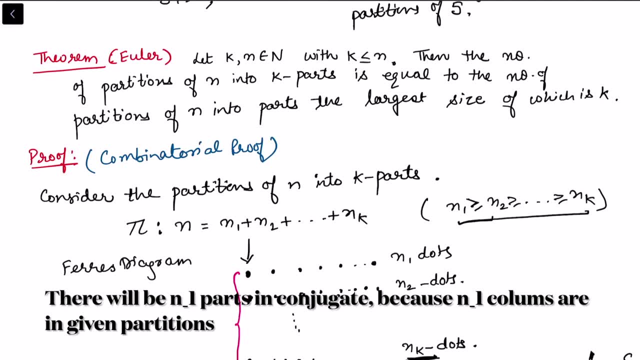 so we do not bother how many parts are there, because the identity says: now, if i look at the identity, it says it partition of n into k part is equal to the number of partition of n into certain parts. it is not mentioned into how many parts, but the condition is that the largest part 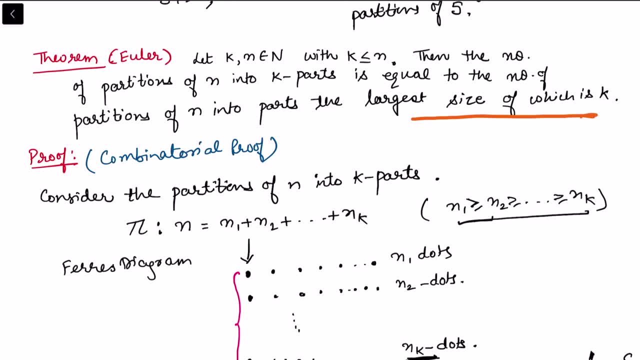 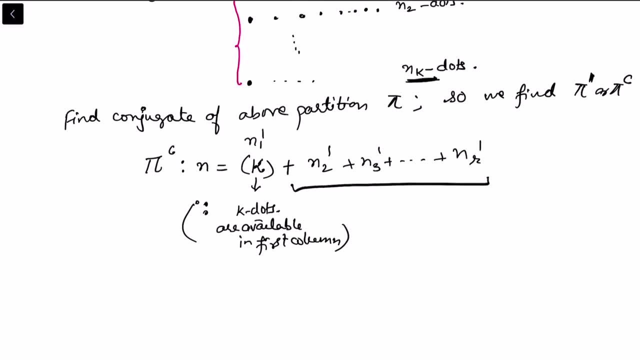 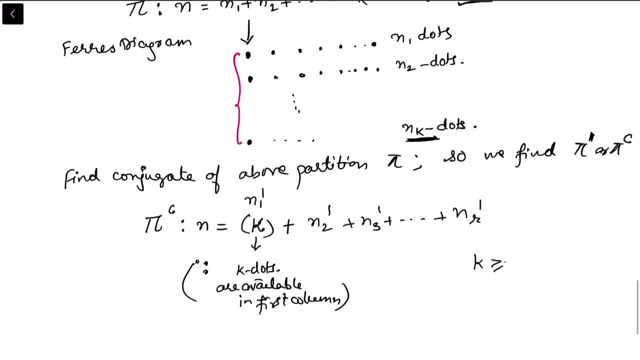 size is of the type of, is of k, or we can simply say: the largest size is k. so this is a partition into some parts where the largest part is k. so the only thing that we know, when you read it vertically, that k is definitely greater than or. 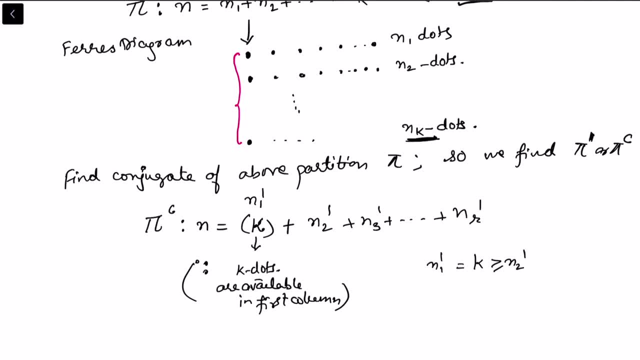 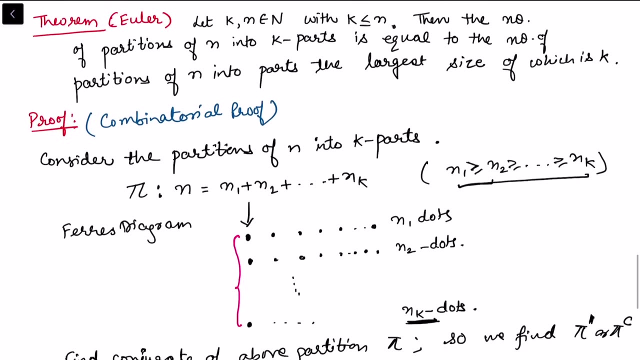 equal to n2 dash. now k is actually the value for my n1 dash, and this is greater than, equal to n3 dash, greater than or equal to, greater than or equal to nr dash. and hence, by the simple explanation or simply taking the conjugate of the fairer diagram, we see this identity holds true and we also see: 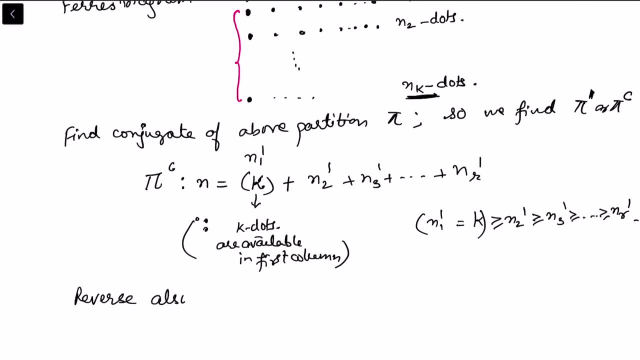 the reverse implication: reverse also hold. so when i what do i mean by reverse? also hold means if i consider a partition in which the largest part is k and then i start reading vertically, so in this case say we have largest part case, so suppose this is there are k dots. now when i'm 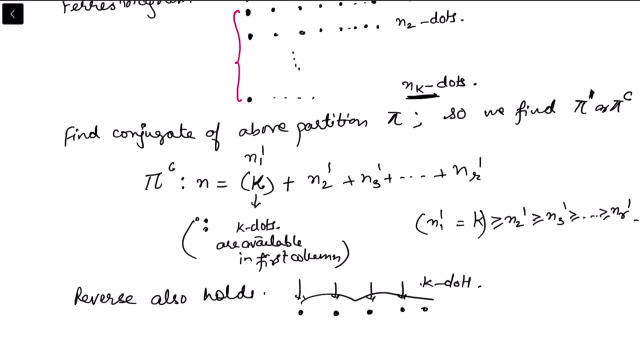 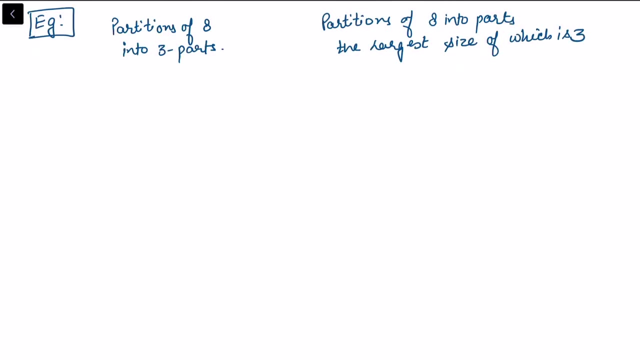 going to read it vertically, that means there will be k parts in that next conjugate of it. so the reverse holds from again taking the conjugate, and that's how we can prove this identity combinatorially. now we see this from this quick example: partition of eight into three parts is equal to partition of eight into parts. 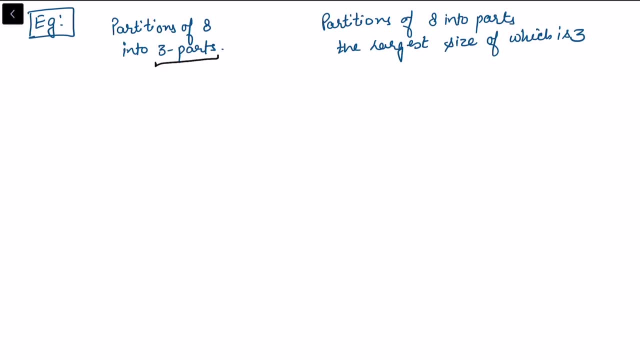 where the largest size of which is three, because here i've considered three parts, this means the largest part size is three and this number, here, this number is same as this number. this is why we are calling it as a partition identity. so now to see this, suppose i consider a partition of eight. 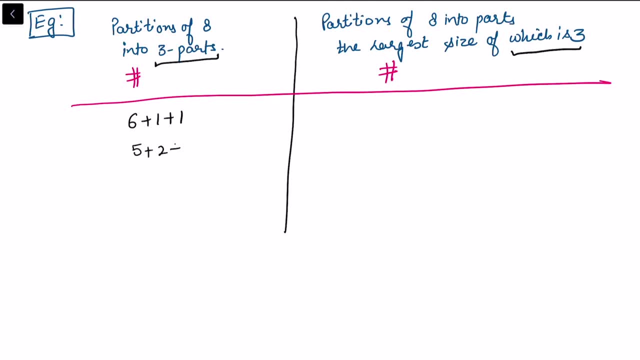 into three parts: six plus one plus one, this is five plus two plus one. here i consider four plus, this is four plus two plus two, and i consider three plus three plus two. now, if i draw the ferrous diagram corresponding to the first case, six one one- we know that the partition will be: 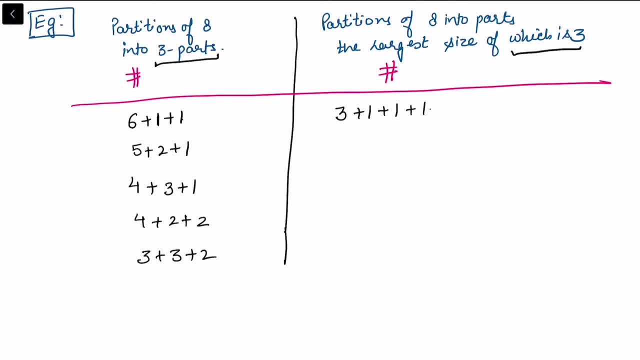 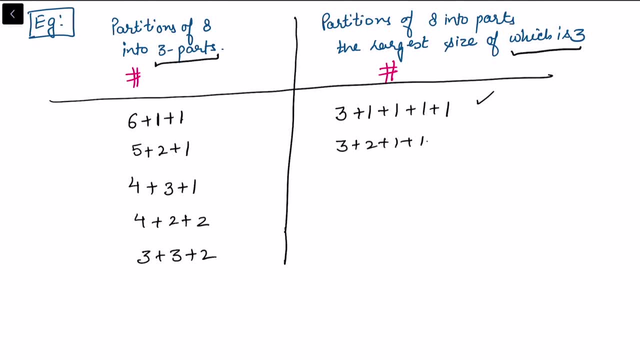 one will correspond to three plus two plus one plus one plus one. four plus three plus one will correspond to three plus two plus two plus one. so this is how they will translate into one another: four plus two plus two. for this also i'll show you four dots in the first row, two dots in the second. 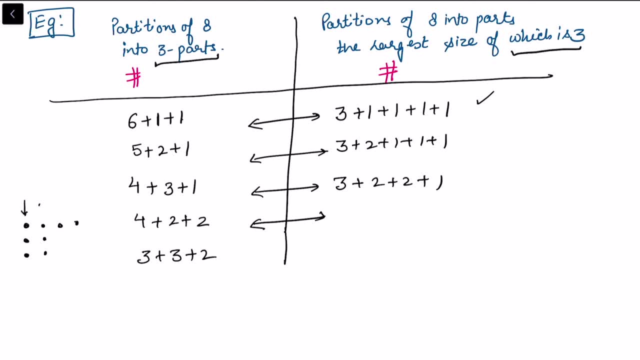 row, two dots in the third row. read it vertically, and so this means four dots in the first and, sorry, three dots in the first, one and three dots here, and then one dot and one dot here. so in this case we will have 3 plus 3 plus 1 plus 1, and then for the last, 3 plus 3 plus 2, we get the partition. 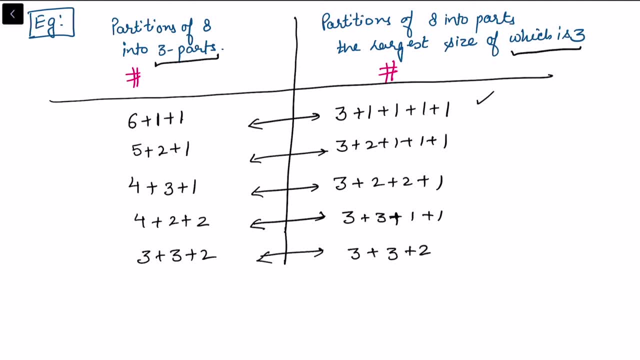 in this case it will be 3 plus 3 plus 2. in fact this one we can call it as a self conjugate also, so this partition is exactly turning into the same partition after the conjugate. so we can consider this as a self conjugate partition and to see the reverse implication. 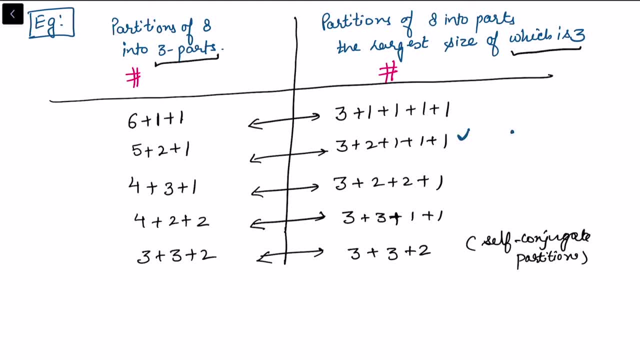 let's say, consider, I am considering this partition, so draw the ferrer diagram corresponding to this. one three. then there are two dots, then one dot, one dot, one dot. now, if I read it vertically, how many dots are there? we can see there are five dots. how many dots are there? there are. 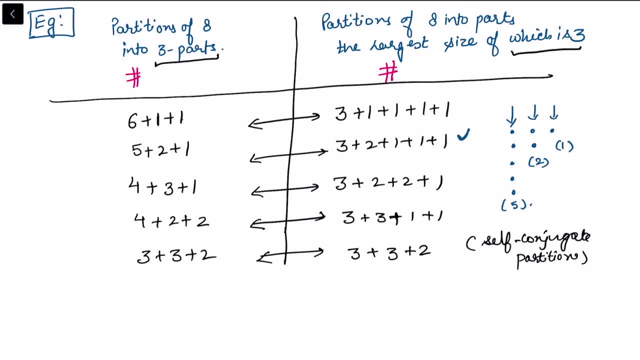 two dots, and how many dots are there? there are one dot, so this is five two one. this is the partition which is listed here, five plus two plus one, because the largest part is three. so in the first row there will be three dots only and these column will become the number. 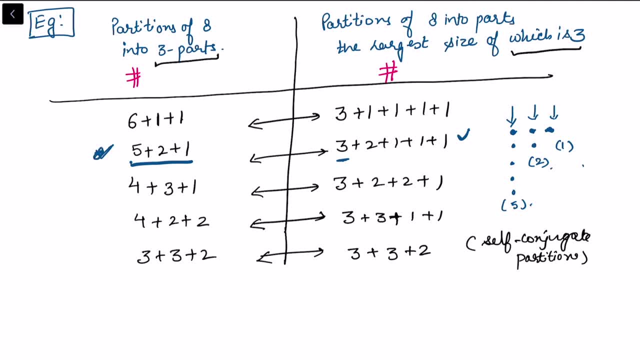 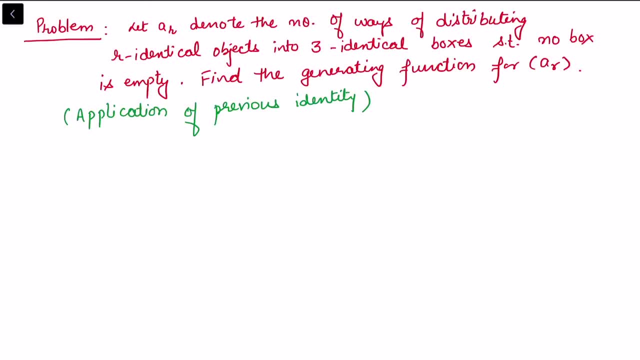 of dots here. so this implication is reversible and hence our identity follow, which is very evident from this particular example. now consider this problem, and this is an application of the previous identity. one can see that, using the previous identity that we have proved one, we can solve this problem very quickly. 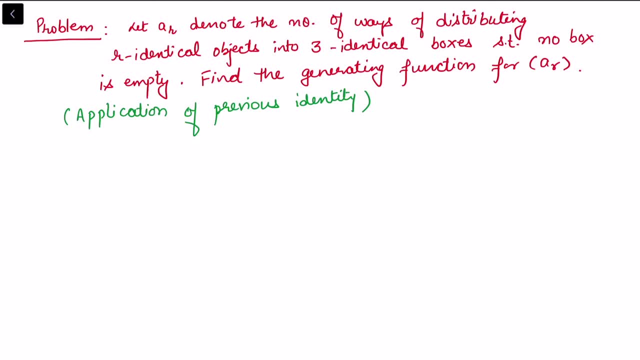 Let AR number of ways of distributing r identical objects into three identical boxes such that no box is empty, find the generating function for AR. so in my one of the previous video I have solved this problem using the generating function- r identical objects into n identical boxes, and there I have shown that this problem is. 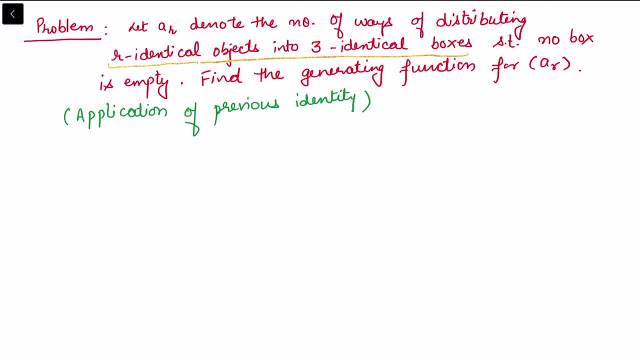 equivalent to writing the number of partition of a positive integer, n. so let's recall the whole. the link is added in the description, but quickly I want to recall all the contents in this. for example you have: n is equal to 3. the relevant partition for 3 r, 3, two plus one plus one. 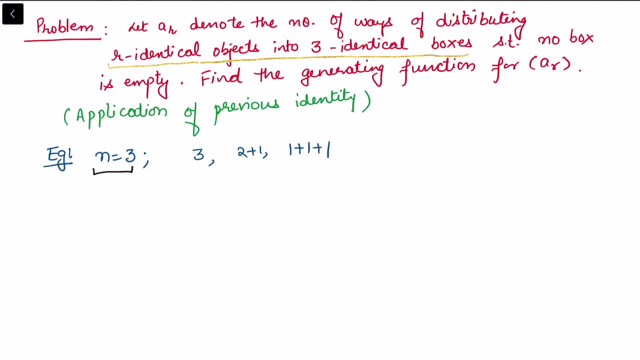 one plus one. so this means if you consider n is equals to three, we need to consider the distribution of the object into three identical boxes, and so for this one we will consider three equalians. you can say identical boxes, and if the part value is one, this means all. 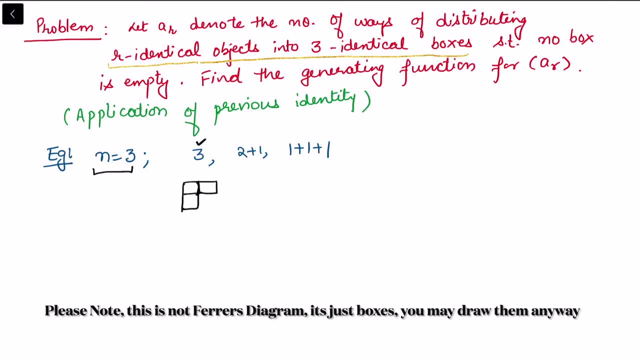 these three. two dots have to be equal or not, assigned only in the one box, because there is only one part. so i will assign all the three dots in the corresponding to this three. the value is three, and so for this i will put up all the three dots in one box. only then, for the next case, how will i assign this? 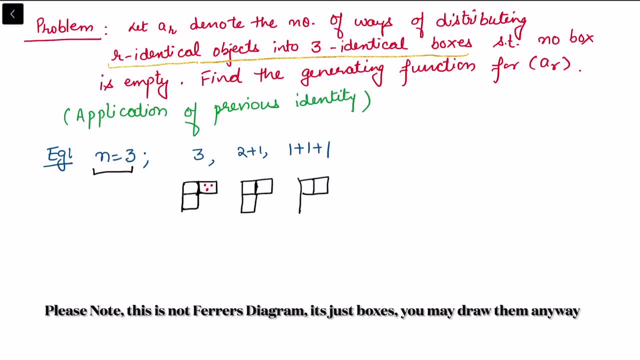 is again into three parts. everywhere this is into three parts. but now if there are two parts, if there are two parts, two and one, the first part have the value two and the one part have the value one. so two dots will go in one box and another n2's value. so this: 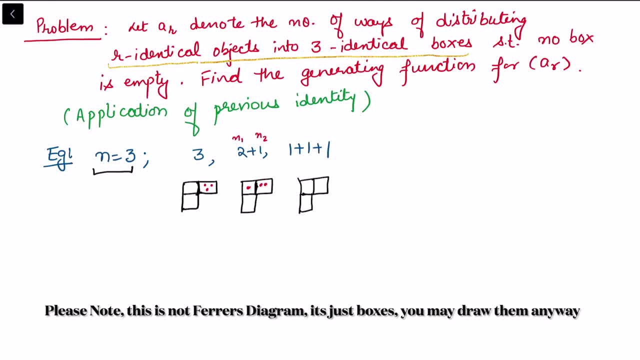 is the value for n1. this is the value n2. n1 goes in one of the box and n2 goes into the another box. then we have 111, so we will place 111. so there are three parts. that means every box have at least one dot. now this is the problem of distributing our identical objects. 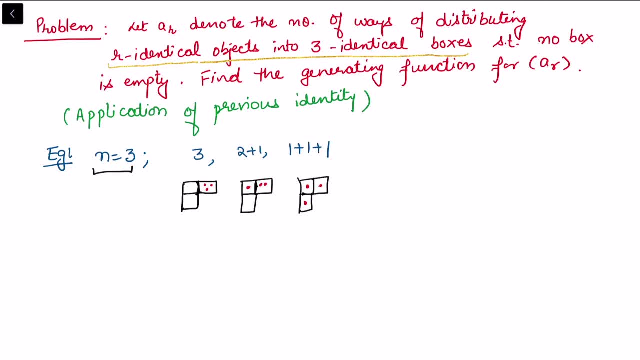 into n identical boxes. when i am explaining this to you, r and r are different. now, same thing, suppose i hear the condition. it says that no box has to be empty. so this means these cases are not allowed, because we can see there are two box which is. 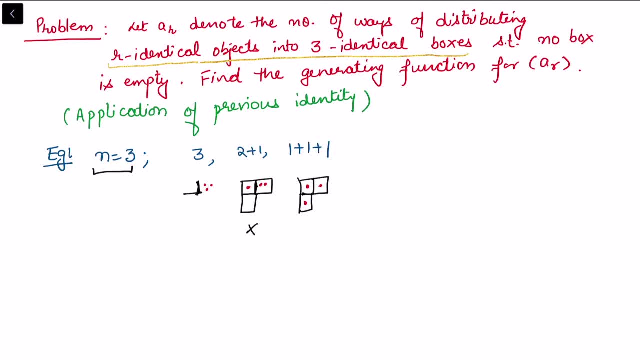 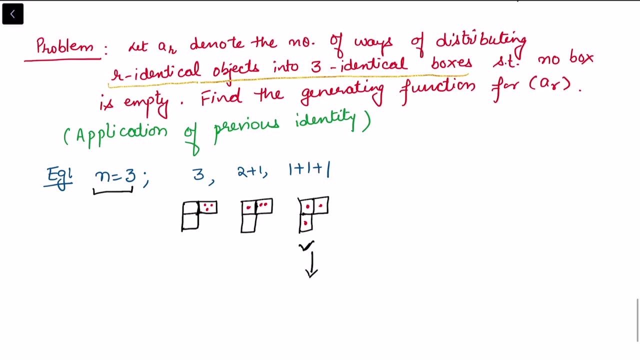 empty. here, one box is empty. this means what our problem is saying. our problem is saying that we want to consider a situation where every box contains at least one object. so this problem: 1 plus 1 plus 1, this case- this is equivalent from the previous understanding. this is equivalent to: 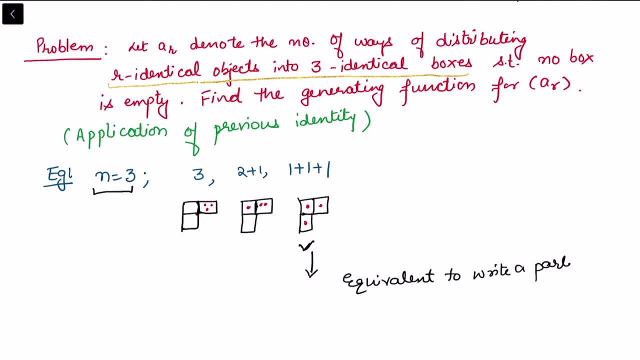 write a partition, write a partition with the largest part, 3, with the largest part as 3, because when i take its ferres diagram, so if i take conjugate of this partition, so what i will get first, i will make the ferres diagram, which is the partition i will get. it's going to be 0 and i'm going to take the partition. 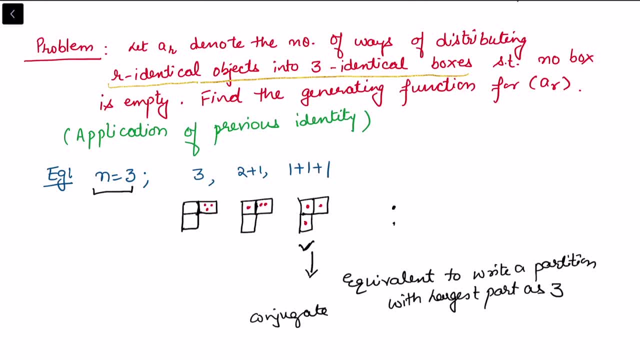 which is the largest part of this partition, and i will make a partition for 2, because is one, one dot in the first row and one dot in the second row and one dot in the third row. so this is the pi partition, which is one plus one plus one of three, and if i just read pi conjugate: 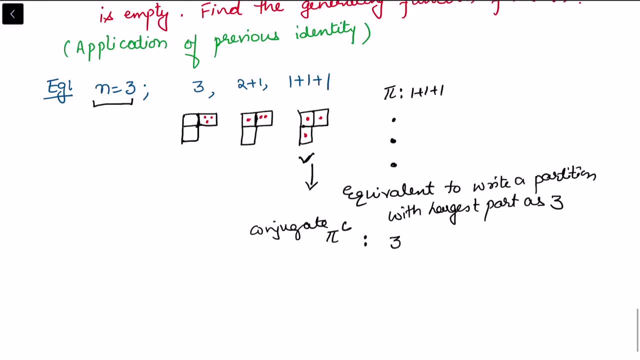 i will get a partition which is three. so this means this type of the things we are searching in which there are one, one, one, one dots. so, for example, if i consider a general case, n is equal to n, this means i am writing a case one plus one, plus one, plus, so on, plus one, up till n times. so 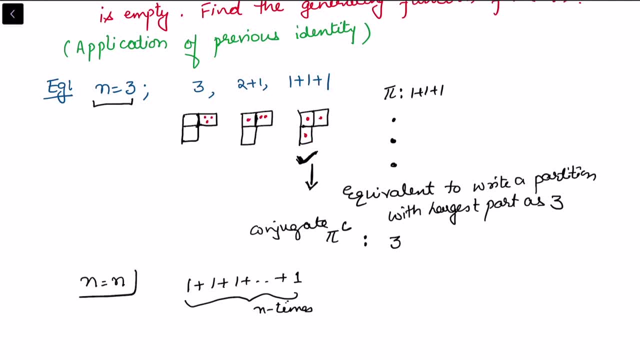 when i consider up till n times, this means when i want to consider a partition of n into n identical boxes. so there are, let's say, n identical boxes and each box has to at least one. so when i consider n identical boxes, every box consists of one dot. so this is what it means now. 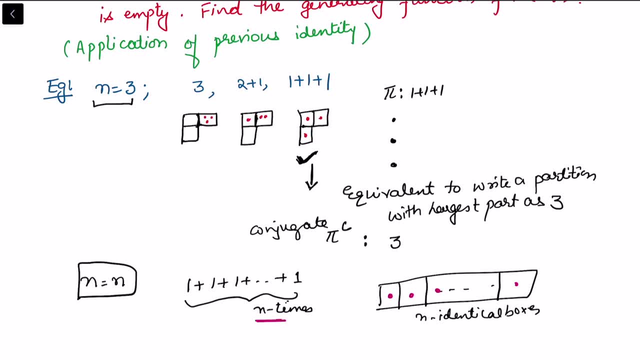 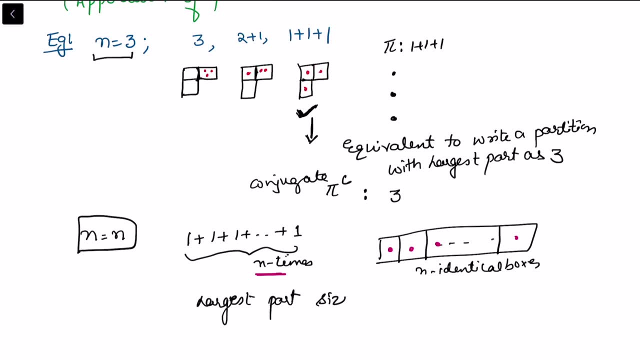 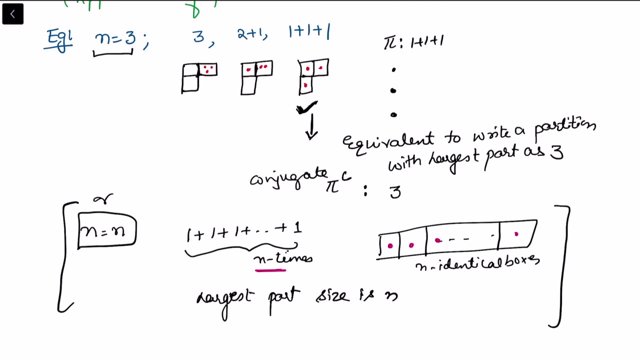 if i consider this case, this is equivalent in solving where the largest part size is n. largest part size is n. okay, so this is what do i mean by the using of the previous theorem. now we will create a generating function as per the part size. we know how to create the. 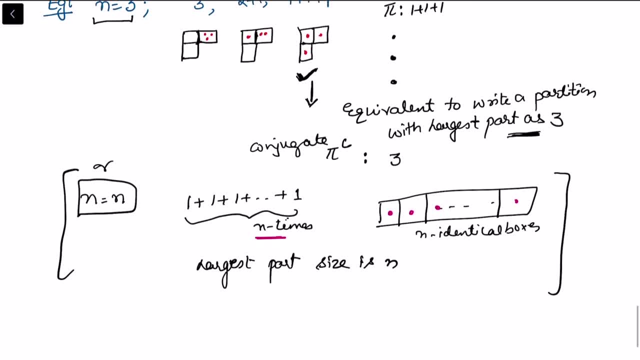 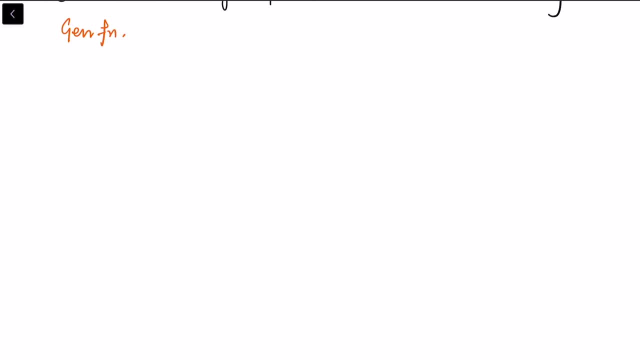 generating function once the part size is known. so for this one now, what i'll do? i'll create a generating function. so generating function. let me to first recall the generating function for the partition integers. recall generating function for pn, this is partitions of n. so we are considering all. 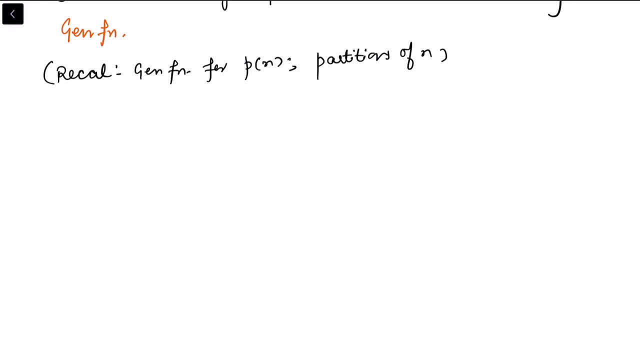 partition of n and here the part size are not restricted. i'm just recalling the previous step. so we said that if the part size is one, x to the power, one may appear or it may not appear. x to the power one raised to power one, then x to the power one may appear twice, and so on. 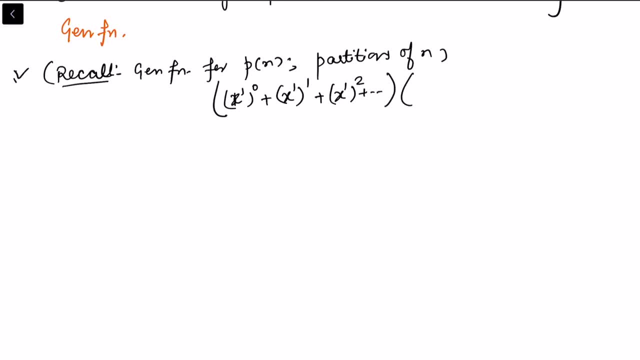 this is the part size one for this particular portion. you need to watch my previous video first, then the part size two can appear zero time. part size two can appear one time, and so on, and this we will repeat for every other part and this is how we written summation pn x to the power n. 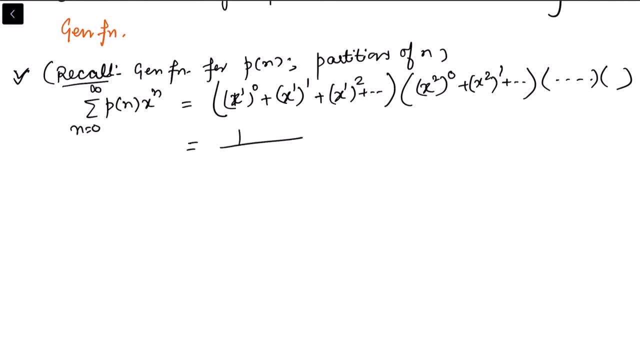 n goes from zero to infinity and then, simply using the gp, we said that this is the part size one for part size two, for part size three, and so on, and so the general function becomes product. so this symbols- i'm using it for product- i varying from one to infinity, one over one, minus x to the power, i so generating function for